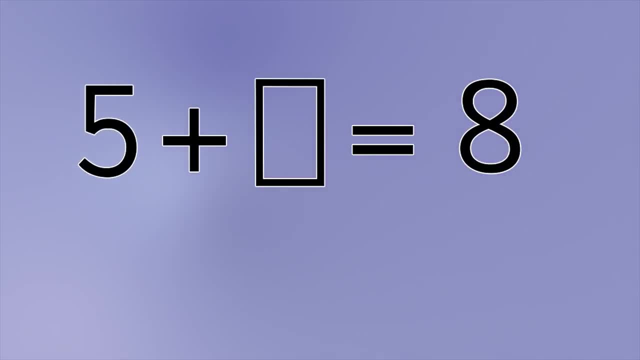 Sometimes a blank box will be used in place of the unknown number, But in algebra, mathematicians replace it with a letter of the alphabet, such as A, B, C, X or Y. This is how they may write it. Five plus A equals eight. 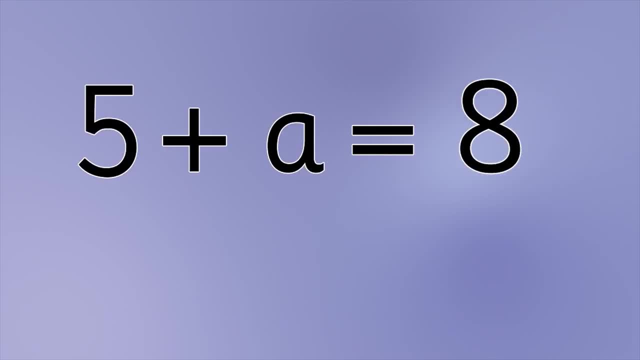 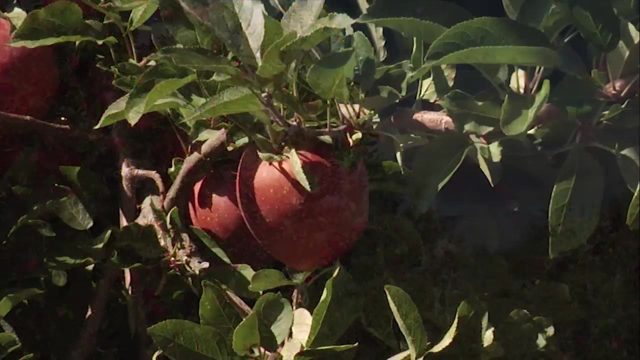 We call this an equation, a mathematical question which includes two parts with an equal sign in between. Now let's look at how we can solve some problems using algebra. Look at these fresh apples growing on a tree. The farmer picks them when they are nice and ripe. 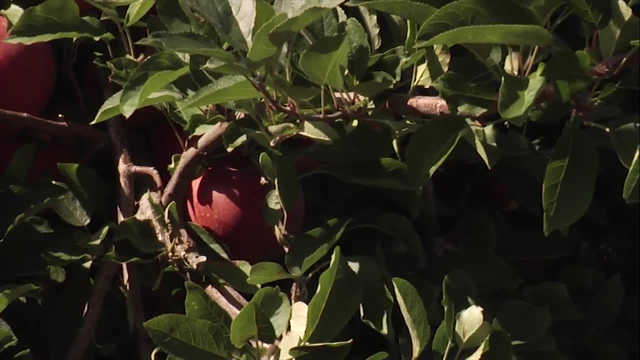 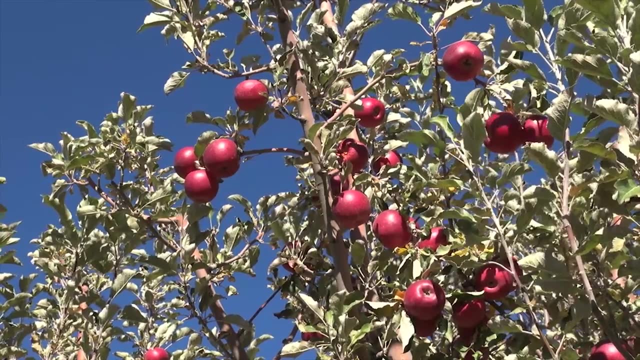 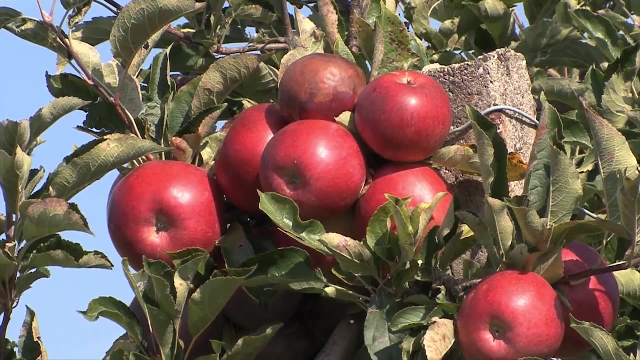 in order to sell them to shops. Some of the apples are ready to be picked. Others need to ripen in the sunshine for a little bit longer. From the first branch, the farmer picked 15 ripe apples, And eight apples were left hanging on the branch. 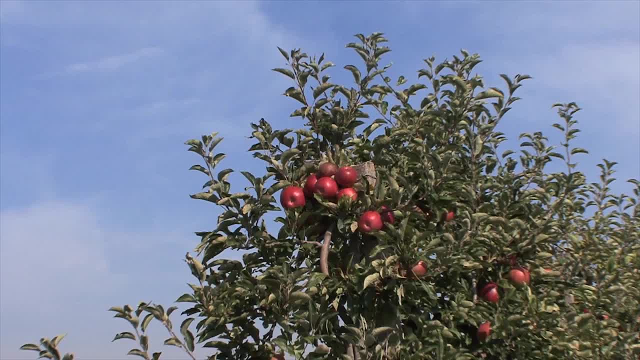 So how many apples were there on the branch to start with? Let's use the letter A to represent the number of apples on the branch. This is how we would write the equation. We started with an unknown number of apples, that's A. 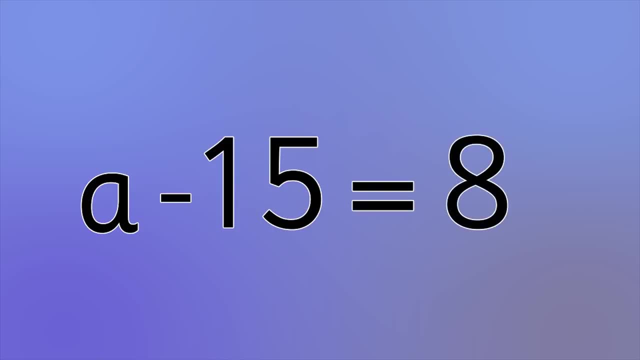 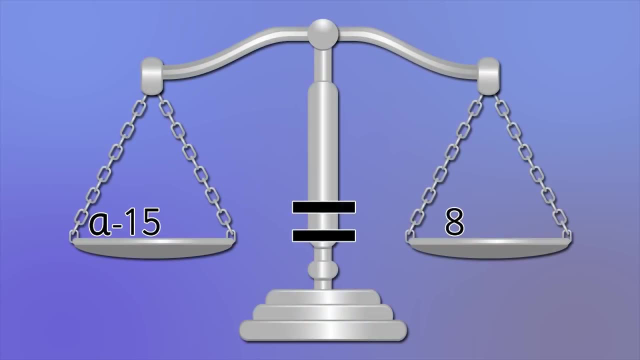 Then we took away 15 and were left with eight. Let's look at the scale to work out the problem. On one side we have A minus 15. And on the other side of the equal sign, the answer 8.. To work out the value of A, we need to isolate A. 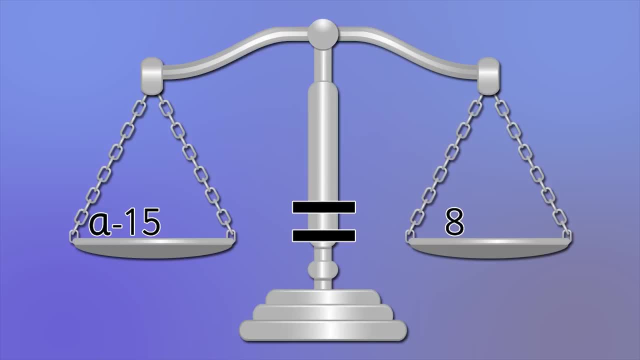 so that it's on its own on one side of the equal sign. That means getting rid of the minus 15.. How can we do that? We remove one operation by doing the opposite operation, the inverse, The opposite of minus 15 is plus 15.. 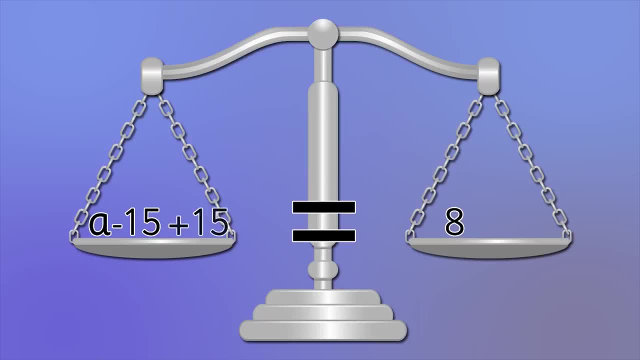 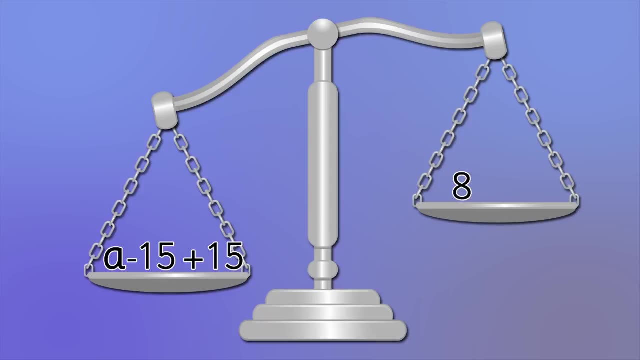 So to isolate A we have to add 15.. But look, that tips the scale. The two sides are no longer the same. For the scale to stay balanced we have to do the same operation on both sides of the equal sign.